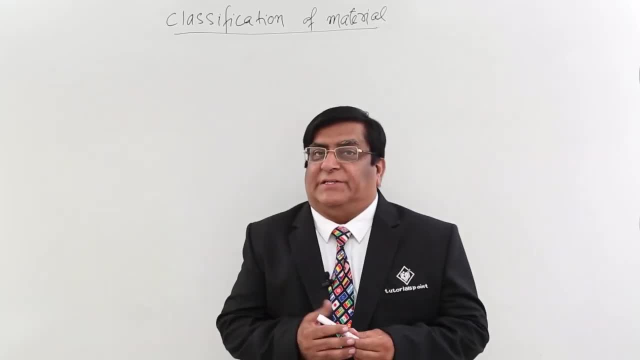 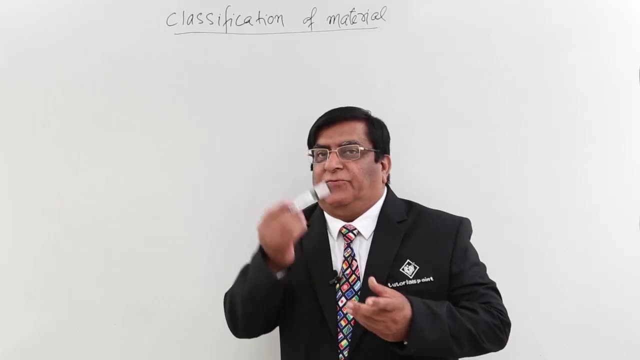 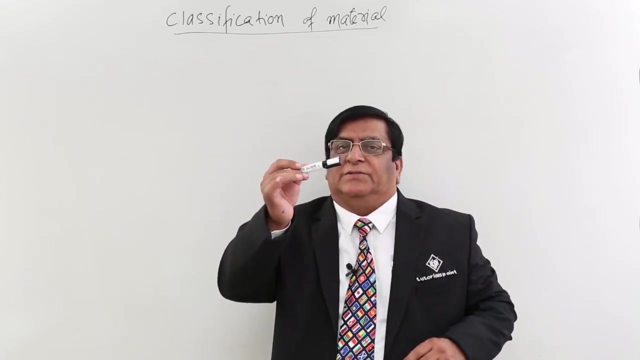 Today we will see classification of material, how we classify material with reference to electric charges. motion Motion means what If I rub this plastic and lift the papers? it will do because it has charged. If I rub a metal plate- copper, silver- then I see: 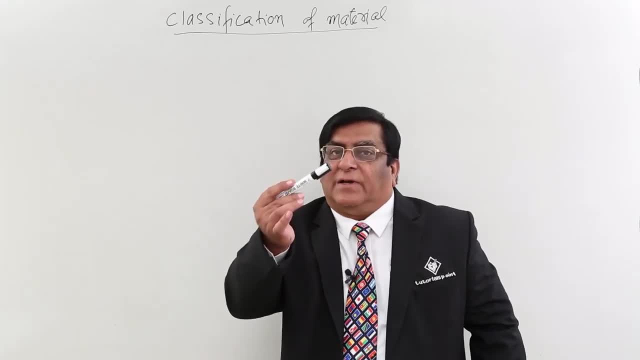 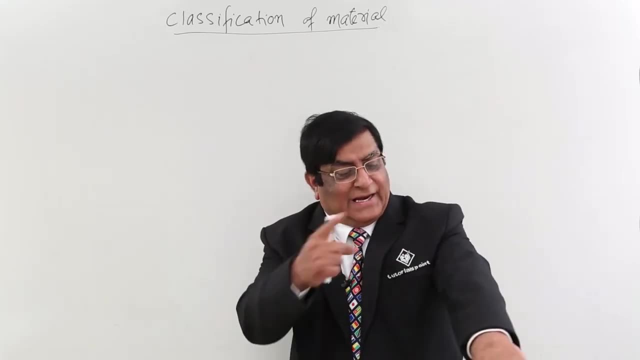 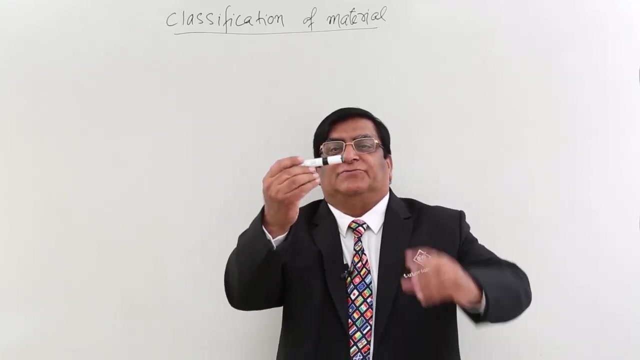 that it is not lifted because? answer: it is not charged, But I am sure it is charged. Why I am sure? Because when I rub it and I check this, this is negatively charged. That means there was a equal positive charge on this. Then why it is not showing the charge? 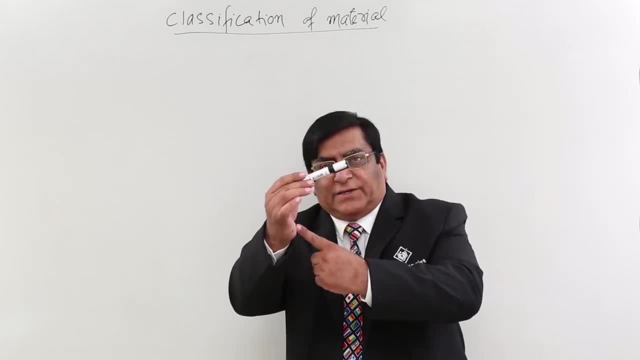 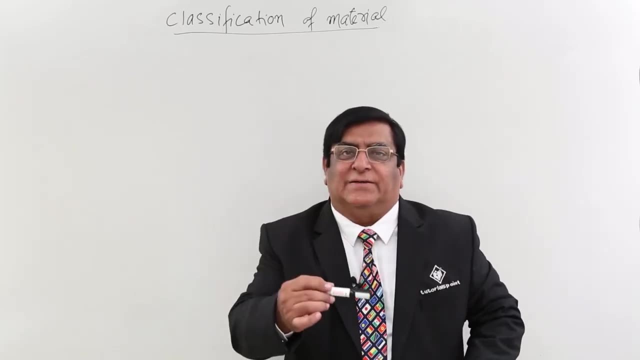 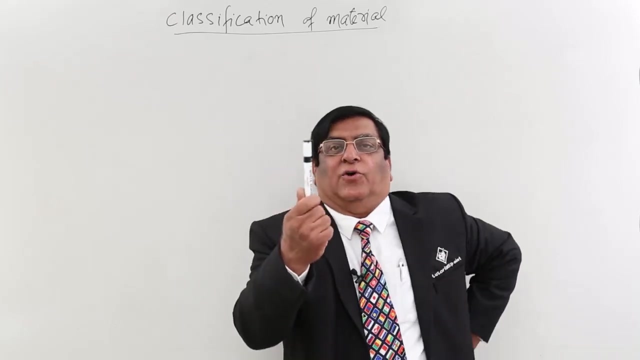 The answer is that charge has gone to my body and it has gone to earth. It should not be happen. every time Now, when I do it with the plastic, it gets charged, and now it is not going to earth. It is showing its force everywhere. Why it has not gone in case of 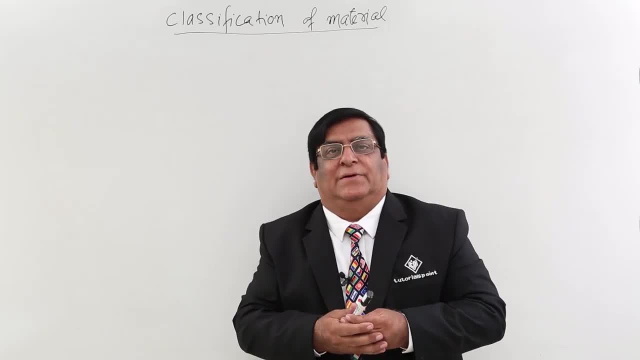 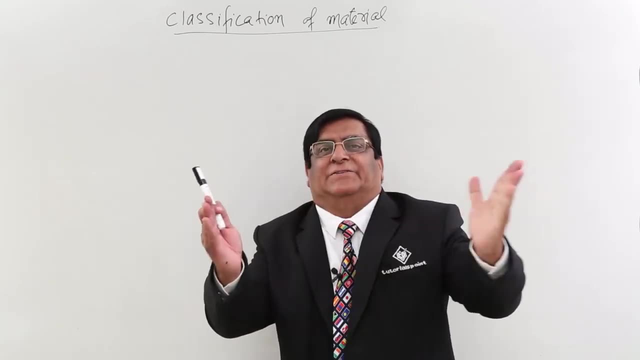 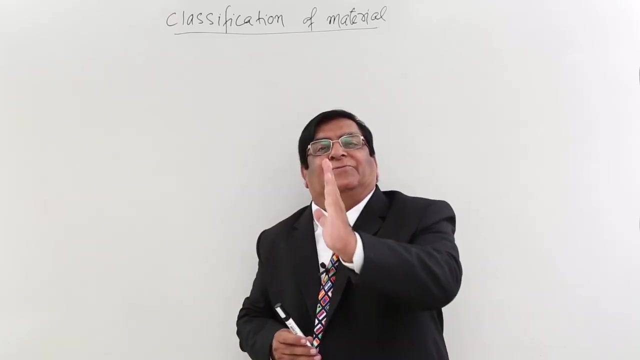 plastic and why it has gone in case of copper, The answer is: we do not have a single answer. and when we do not have a single answer, we classify. Few things behave like this. few things behave like this. The same thing we have done for the material and we classify. 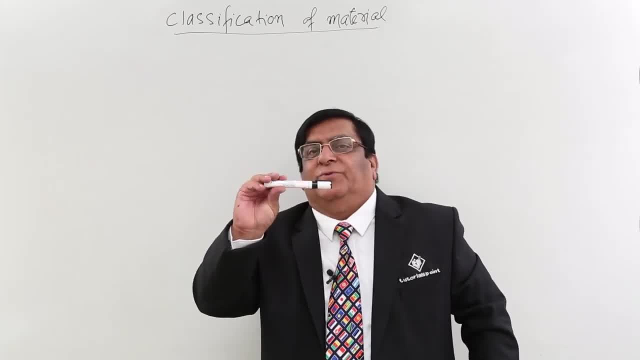 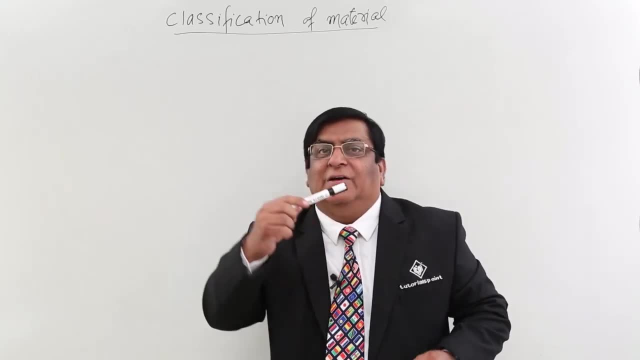 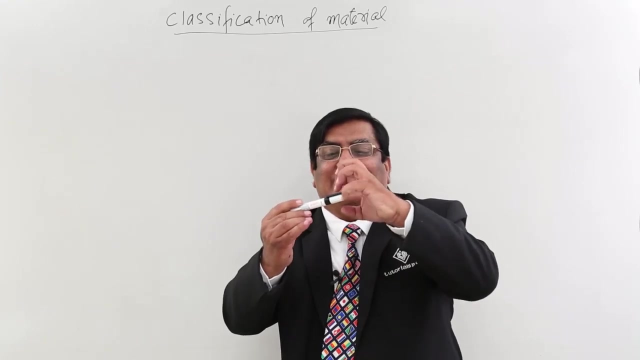 the material. There is one class of material which allows charges to move- copper, silver. There is another class of material which do not allow that to move. that is glass, plastic. You rub it, this particle will get the charges will accumulate here and these charges will. 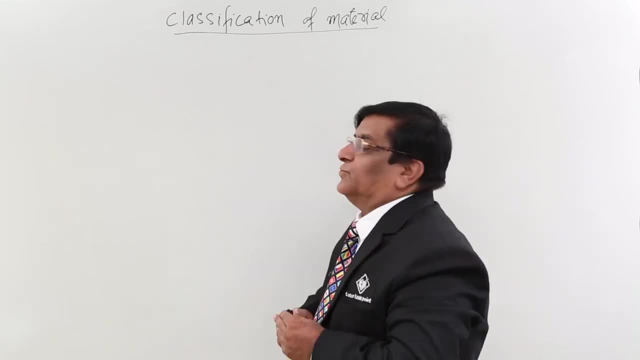 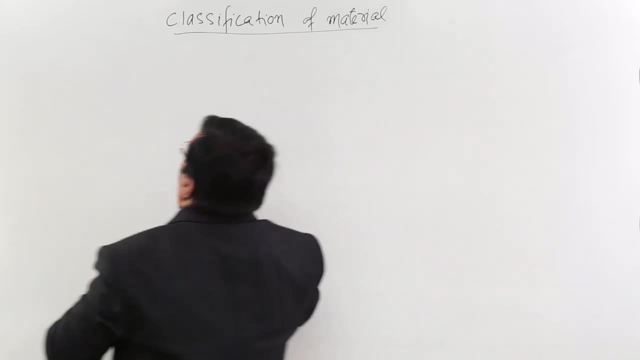 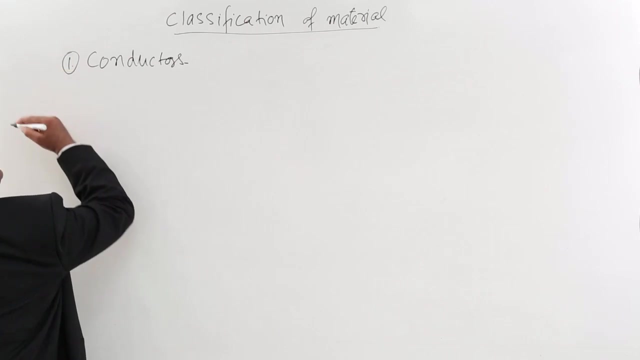 not move. So we classify into two types: one which allow the charges to be conducted. The one which allow the charges to be conducted is called conductors, So we call them conductors, And other is we will call them insulators, Insulator, which will insulate the charge. here. 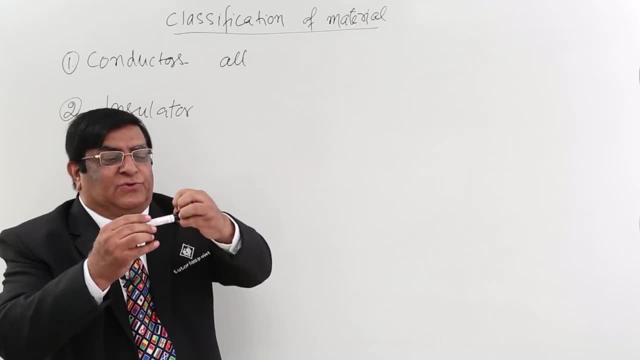 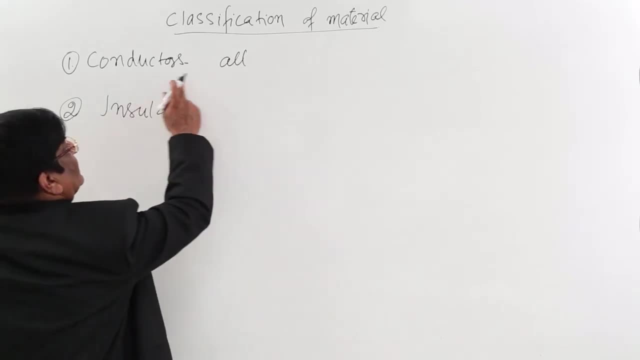 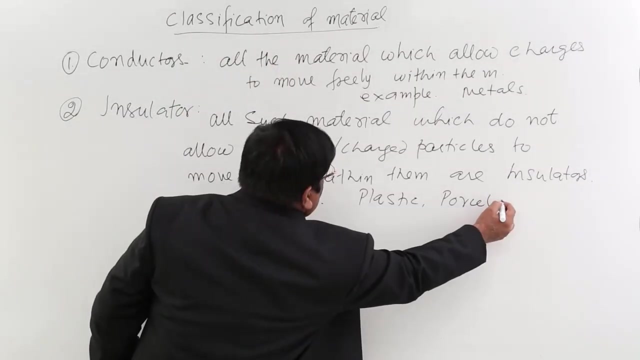 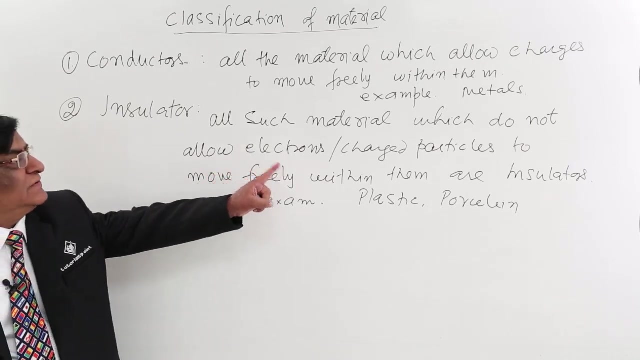 insulate, separated out, So which will insulate the charge on this part, from this part. So conductors are known as insulators, So conductors. I will write the definition of the two Insulators: all such material which do not allow electrons or charge particles to move. 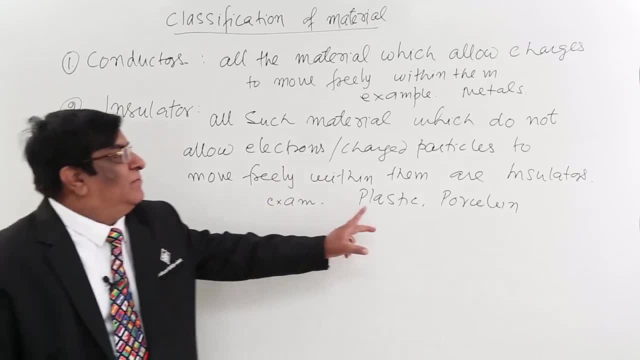 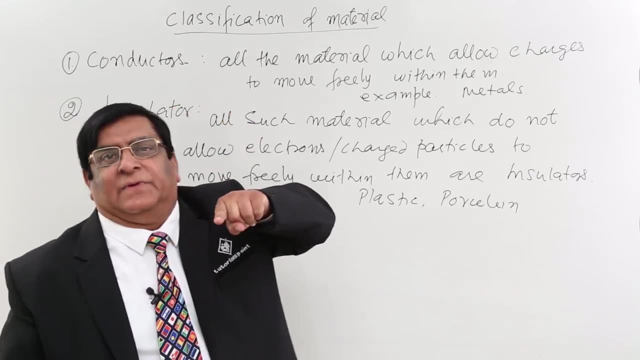 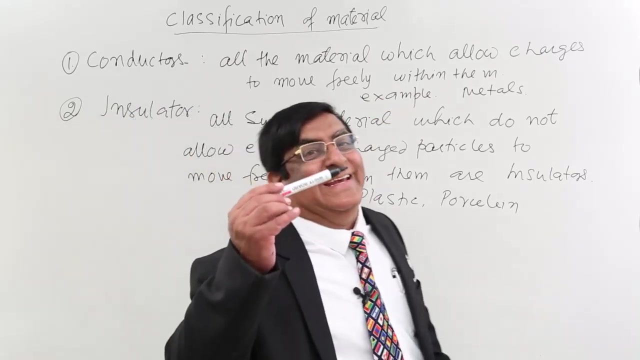 freely. within them are insulator Plastics, porcelain. ok. Now, this property of conductors, which are known as insulators, are known as conductors- So conductors are known as conductors- allows charges to move, makes them conductor. We need it whenever we want to carry charges. 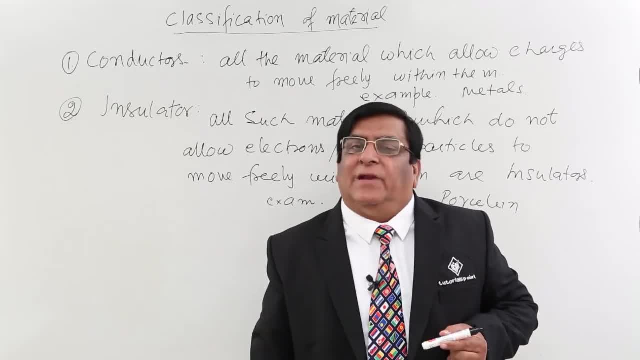 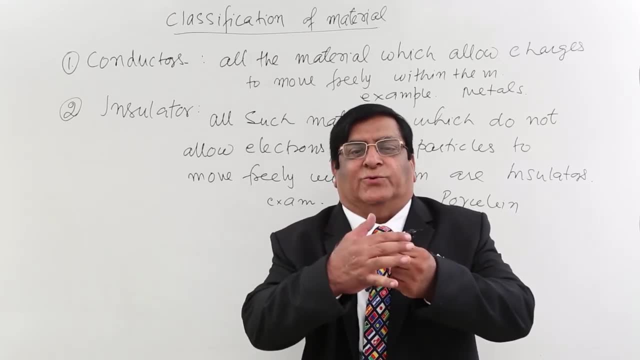 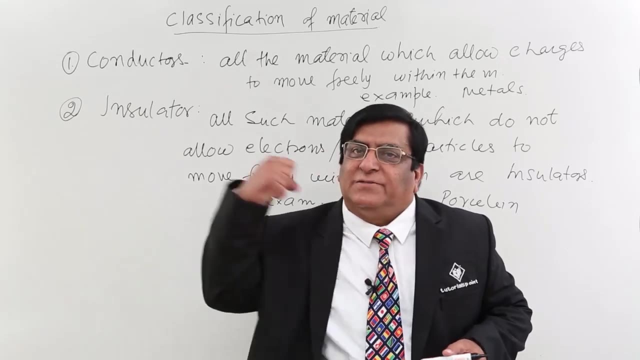 from one place to the other place. We need a conductor. Like the, power house is generating electricity and I need to move charges from power house to my house. So what do I need? I need a conductor. Now I want that all those charges pressed by power house should come. 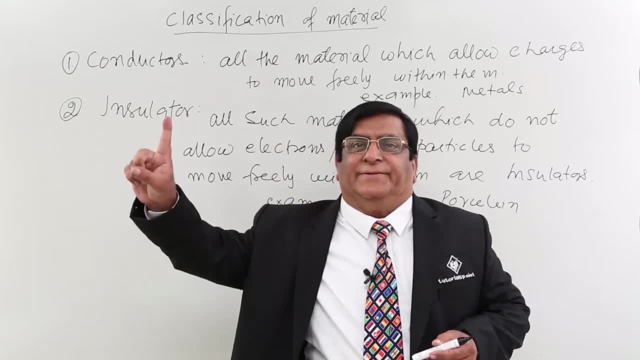 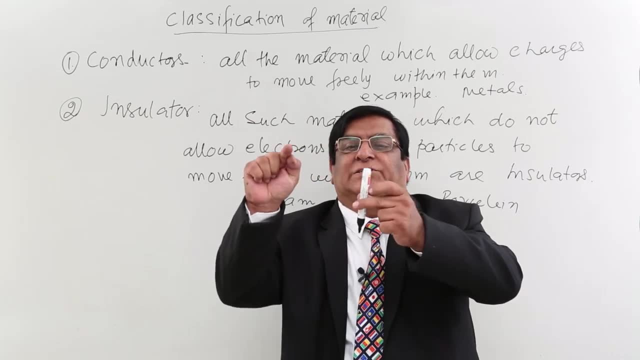 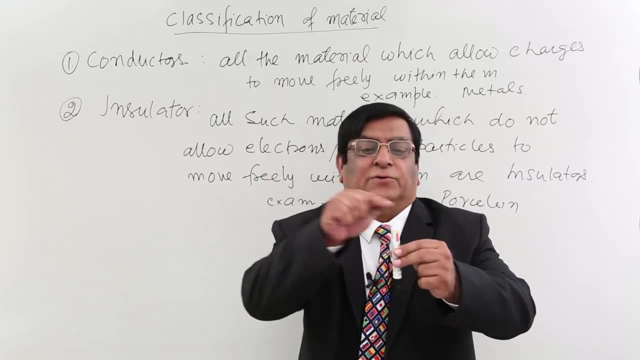 to my house, but such a long wire I have to rest on the poles. Whenever this wire is going to the pole, the charges will come here and will go to earth. I want them not to go to earth. I want them to come to my house. So what can I do to avoid that they should not? 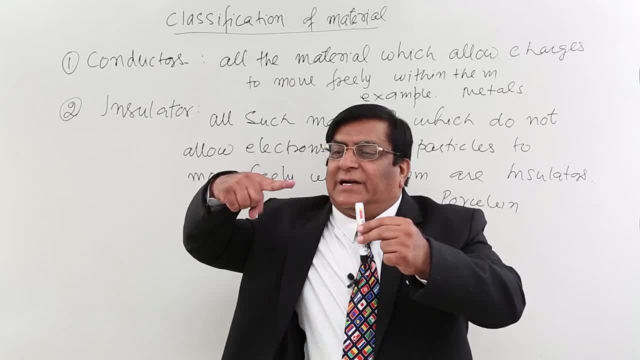 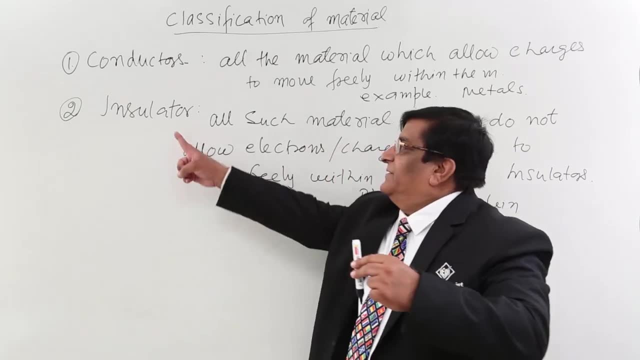 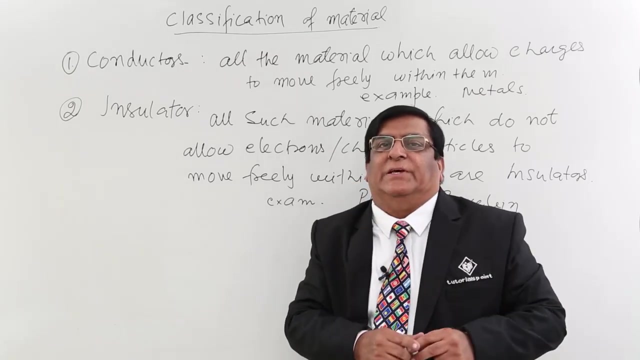 go to earth? The answer is: when there is a conductor coming to my house, in between conductor and this pole, I will put an insulator. What it will do? It will not allow charges to move to this. and this is what you see On the poles. just see it minutely, always you will find. 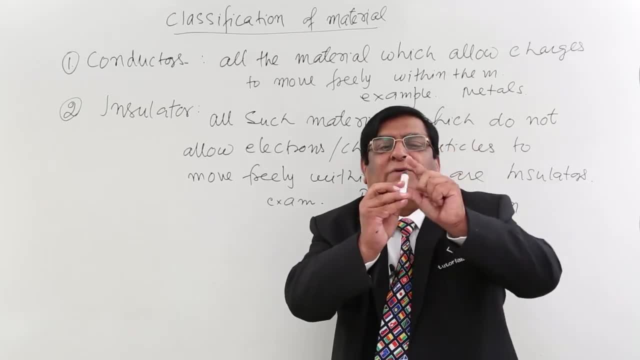 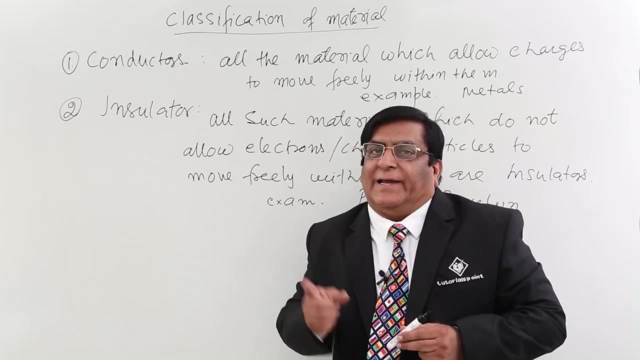 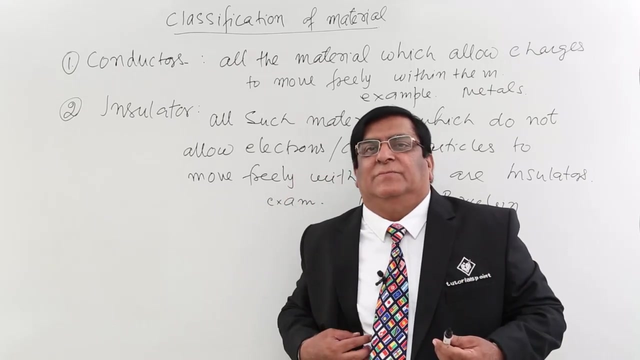 that the wire is not connected to pole and there is always a porcelain between them. That is why we save charges to move Simply again, we do not want charges to move through our body Because that will destroy our nervous system, which is also an electrical system. So charges